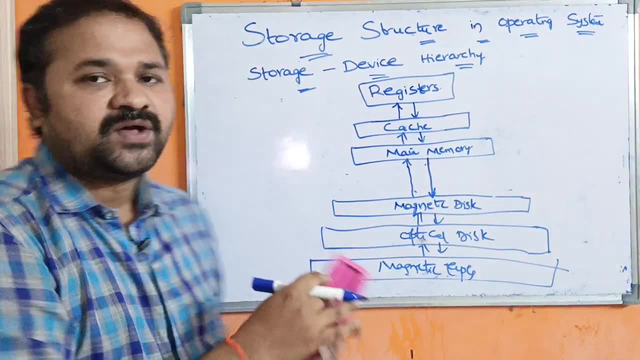 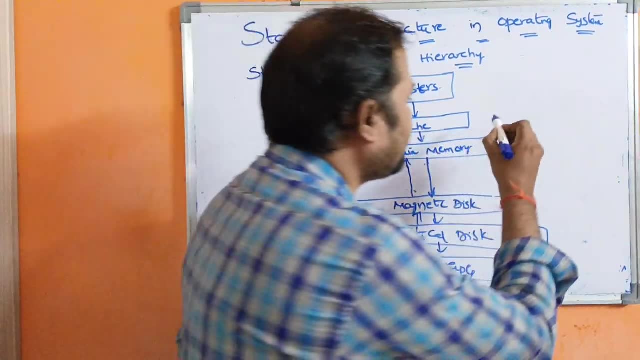 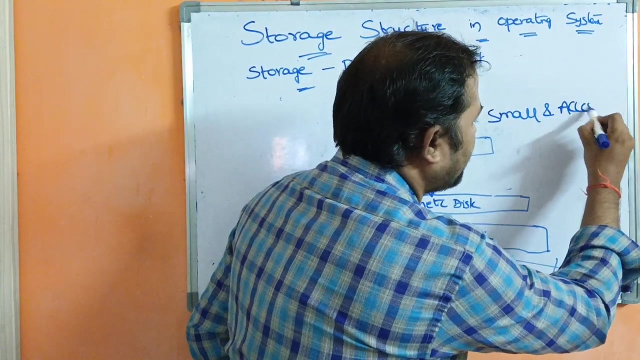 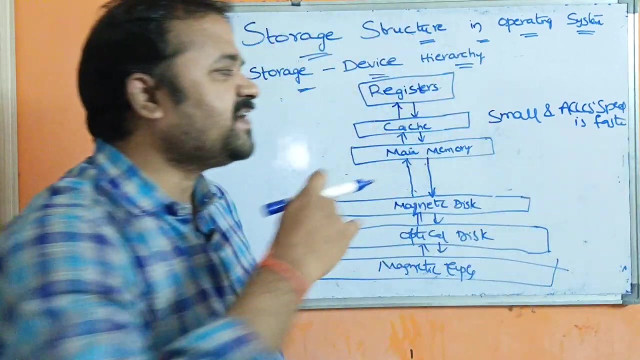 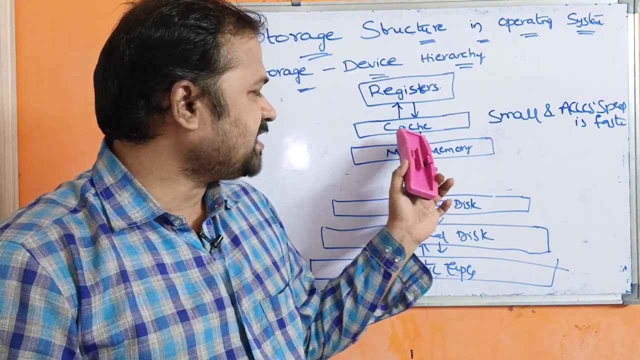 cache memory. cache memory is very, very small memory, but it is very, very faster memory. so what about cache memory? it is very, very small memory, but access speed is very, very faster. access speed is very, very faster. access speed is faster and it is very, very expensive memory also, and it is very, very expensive memory also. okay, now let us see about. 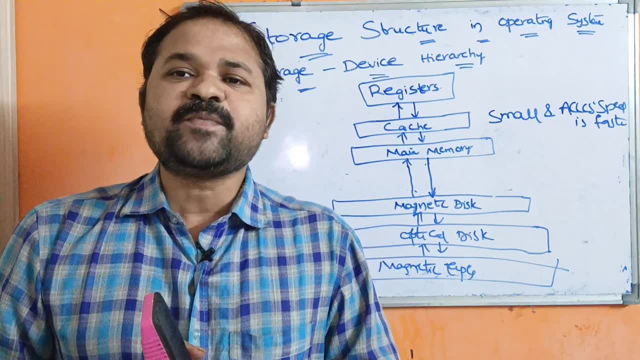 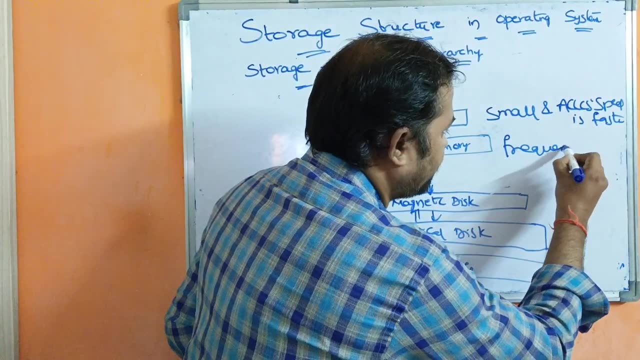 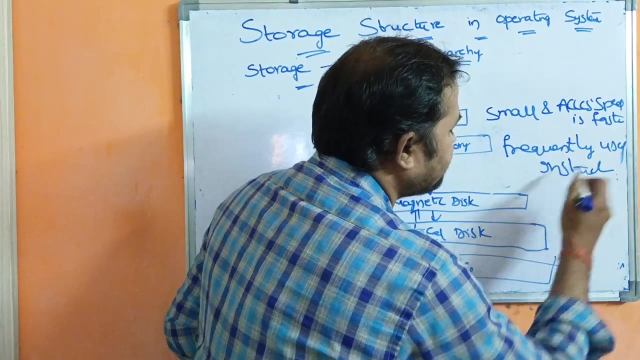 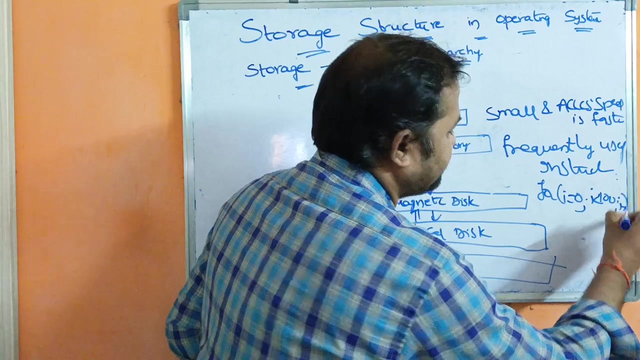 some more properties about the cache memory in order to store frequently used instructions. so cache memory is useful for storing frequently used instructions. let us take the example of a for loop. we have a for loop such as: I is equal to 0, I less than 100, I plus plus okay, so in. 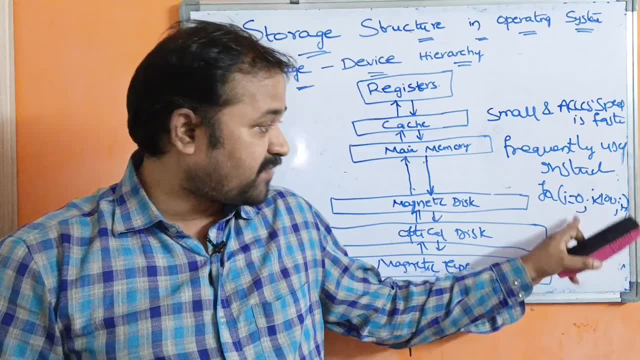 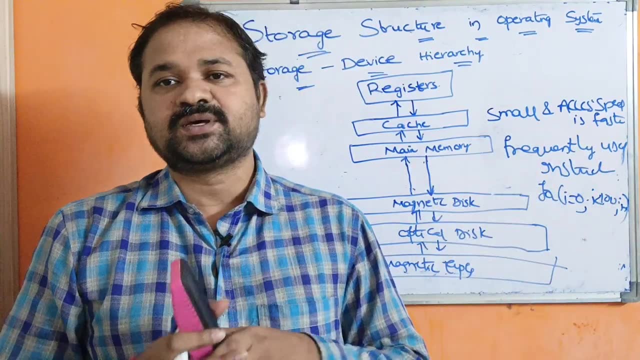 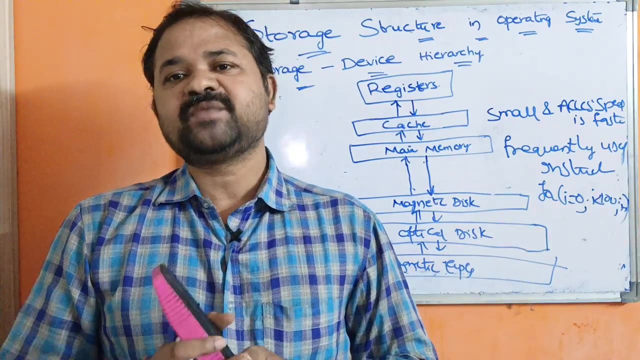 this situation. what we are doing? we are repeating the for loop for 100 times, so that means cpu has to access i hundred times. in those type of situations, operating system stores the data in cache memory by, because cache memory is very, very faster, very, very fast, and I'm and memory okay. 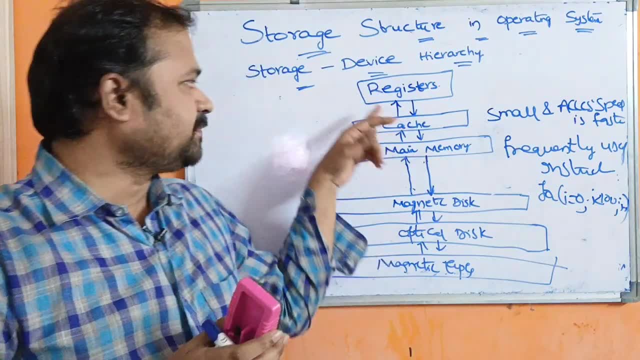 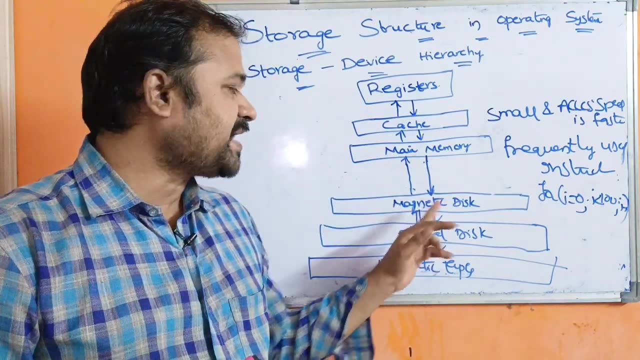 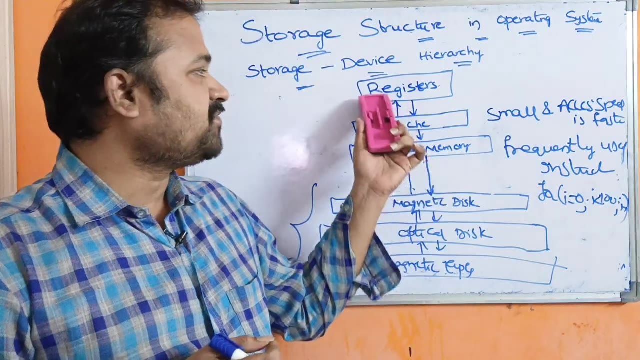 cpu can access the content of the cache memory as well as cpu can access consistent and cpu can also access main memory. but cpu cannot access all designs which i have said in the video we use return. that Doncs you drag a secondary memory devices. cpu cannot access all these secondary memory devices. but here what is? 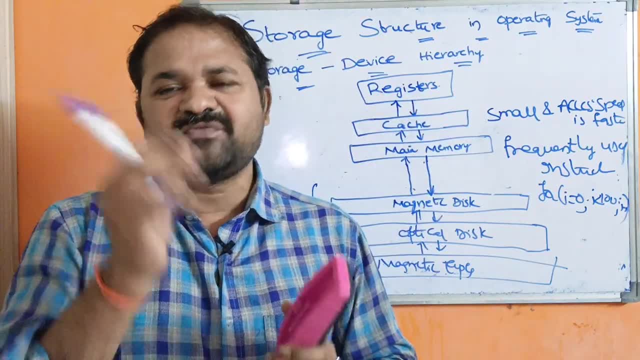 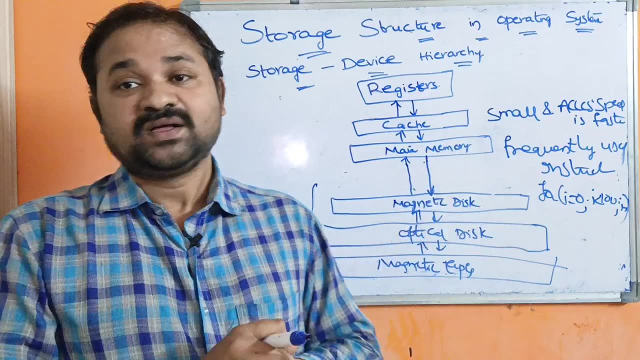 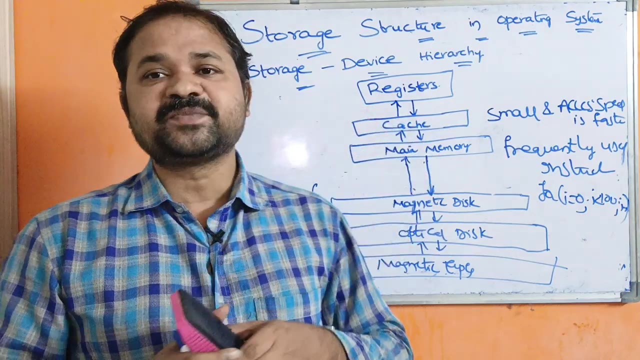 the problem with register. register store only piece of information. it stores 16 bit, 32 bit, 64 bit, likewise only. so if we have a mb of data, then with the help of the register we can't store that much of information. so in the type of occasion operating system uses the catch memory. okay. 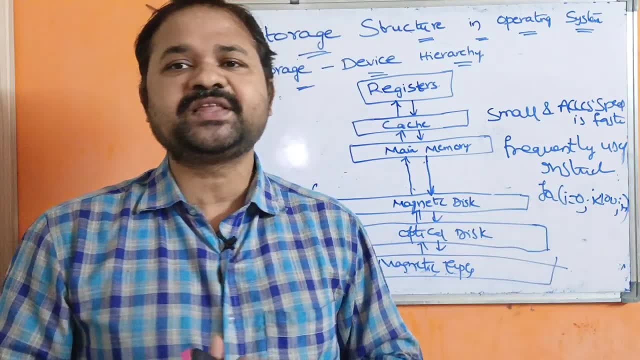 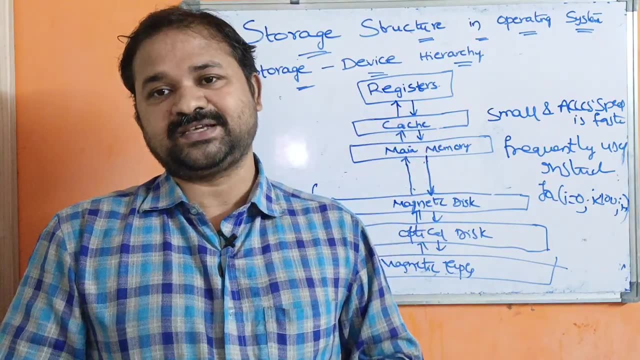 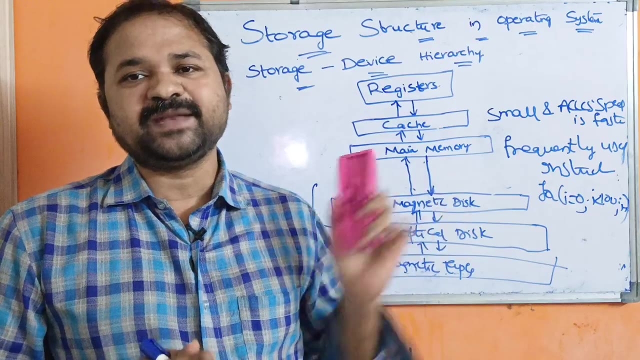 so, uh, so it is mainly useful for storing the frequently used instructions. okay, cpu can access memory content very, very fastly then, if it resides in main memory. now let us see about main memory. let us see about main memory. main memory is also called as primary memory. why? because 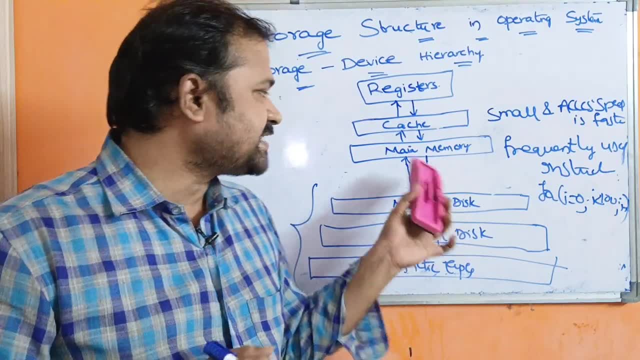 cpu can access the the data if it resides in main memory, main memory generally. you see in the these things that the main memory is being stored in, so it is controlled to gain memorynamename and memory key. hyvinpc, okay, even on you can create a main memory, mainese just. 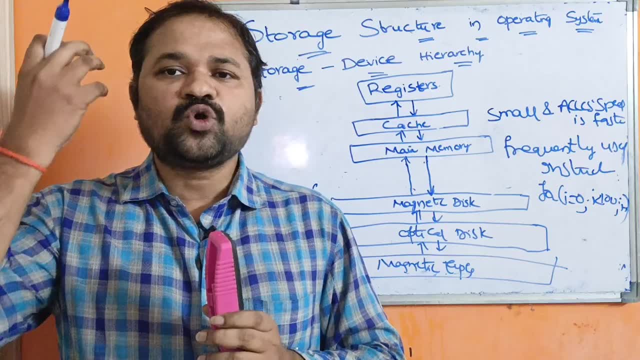 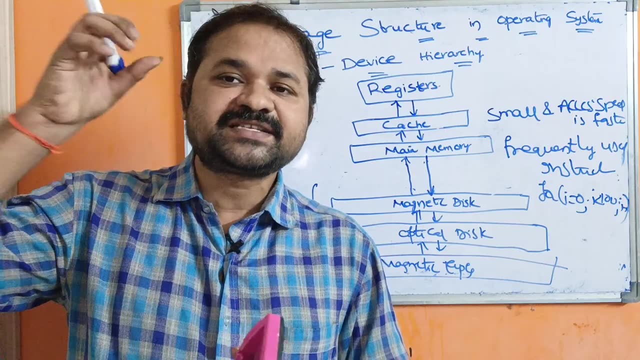 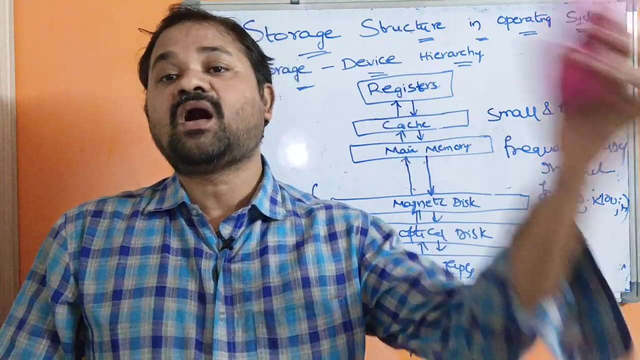 Generally, whenever we save the program, then the program will be saved in hard disk. At the time of compilation also, the program will resides in hard disk, But at the time of execution, operating system transfers the program from hard disk into the main memory. 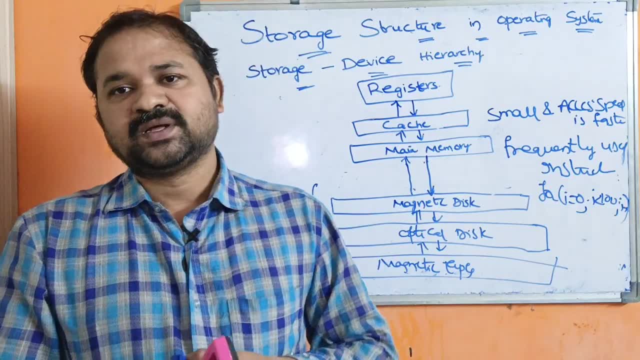 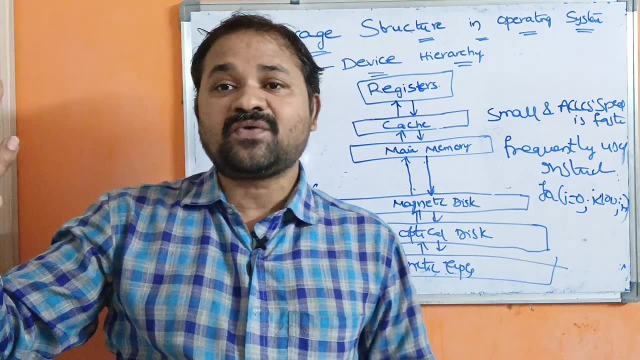 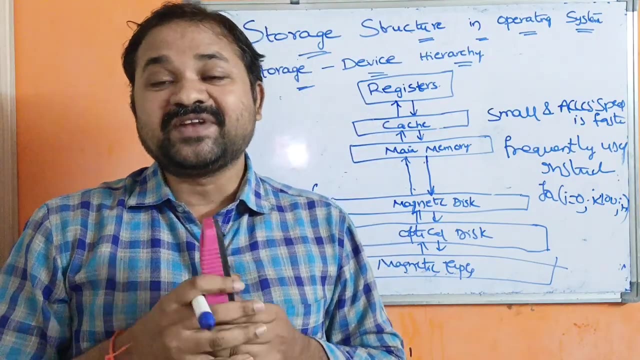 Let us assume that we opened some Microsoft Word. initially it will be in hard disk only, But whenever we double click on that Microsoft Word, then that Microsoft Word operating system loads that Microsoft Word from hard disk into the main memory. So it will transfers that word from hard disk into the main memory. 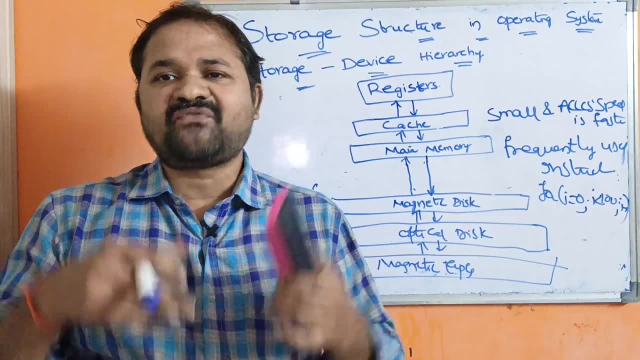 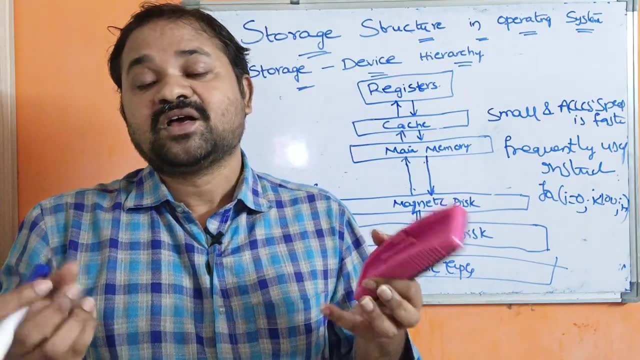 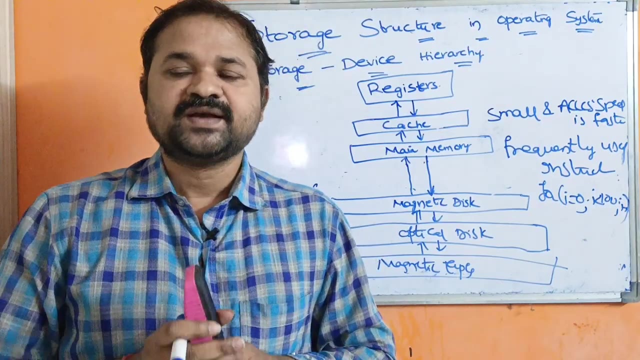 Let us assume that we are watching a movie, So initially, after saving that information, after saving that movie, it will be stored in hard disk only, But while watching, whenever we double click on that video, then operating system transfers the movie From hard disk into the main memory. 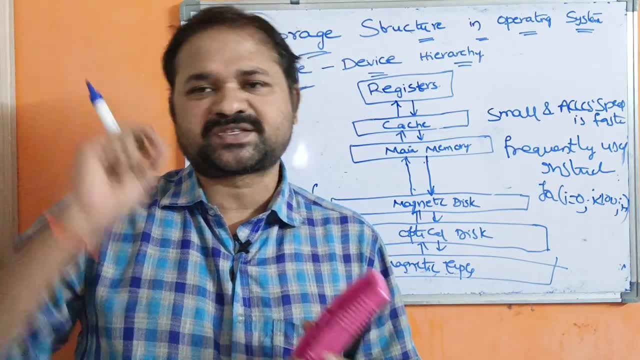 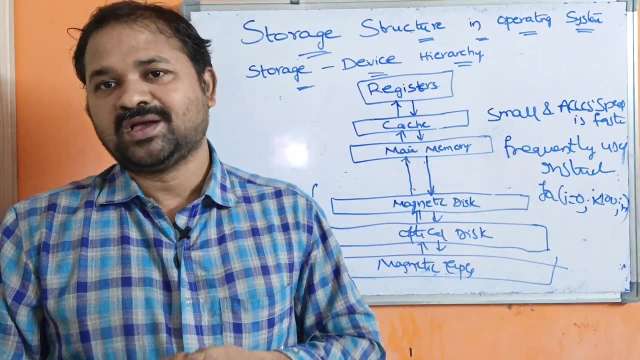 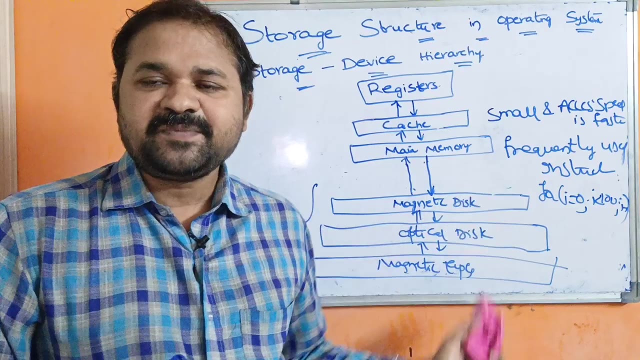 So here the point is: CPU can execute any task if it resides in main memory only. So that's why main memory is called as primary memory. Why? because main memory is very, very important memory. CPU cannot access the content of the secondary memory. 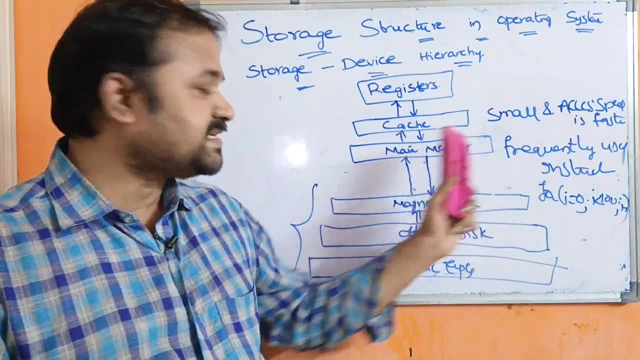 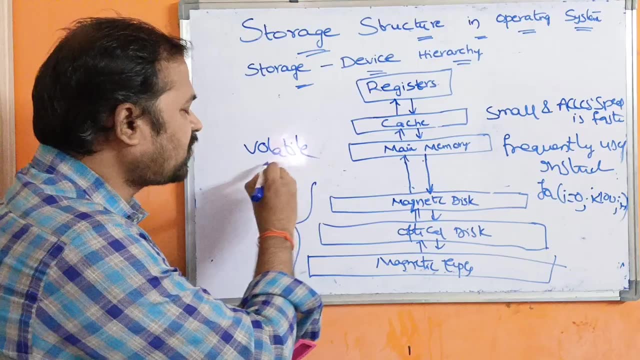 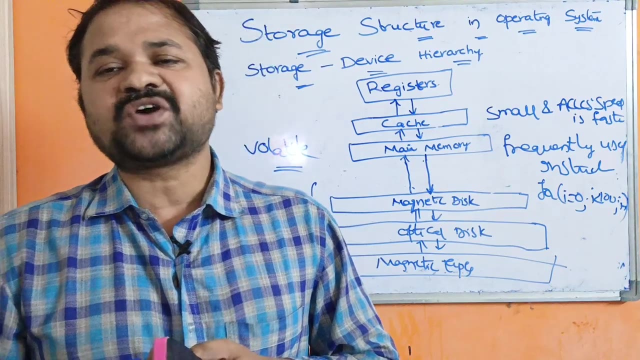 CPU cannot access secondary memory, But CPU can access main memory. Main memory is also called as volatile memory, Because volatile means whenever we switch off the computer. when the computer is turned off, then the contents of the main memory will be lost. So that's why main memory is called as volatile memory. 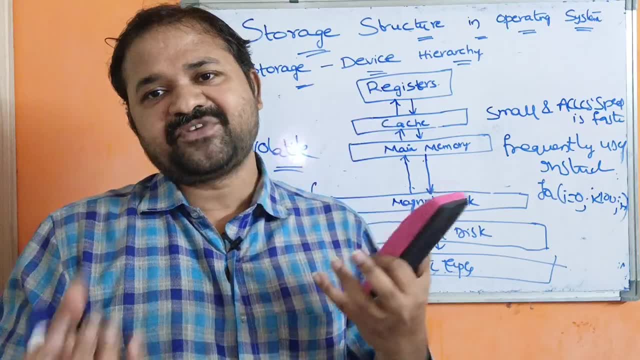 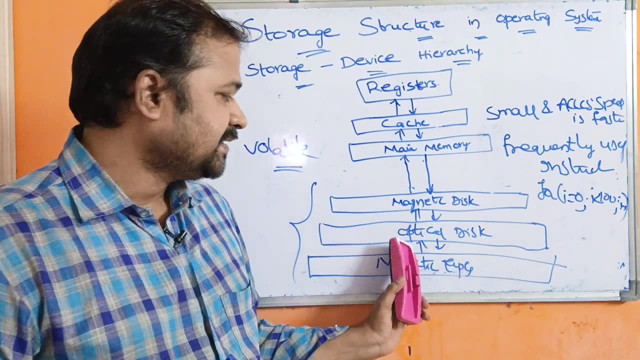 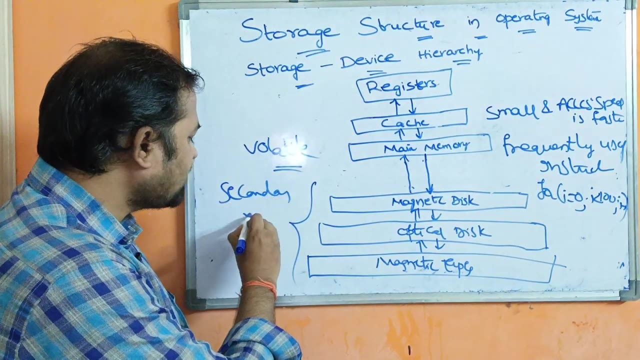 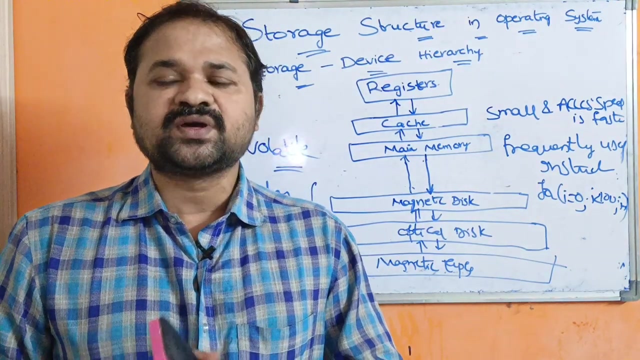 So we should have a memory which stores the information permanently. So for that purpose we use magnetic disk, optical disk and magnetic tape. These are called as secondary memory devices. So let us see about what is secondary memory. Secondary memory is useful in order to store the information permanently in the computer. 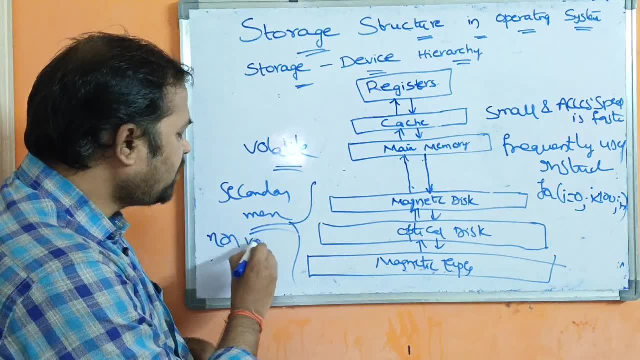 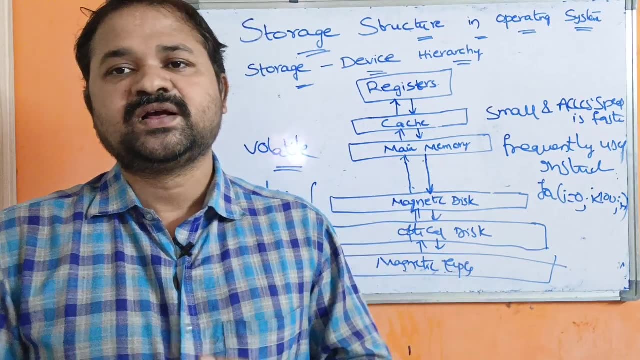 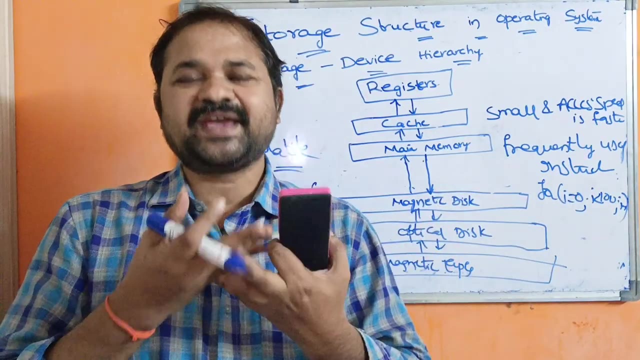 Secondary memory is called as non-volatile memory. So that means when we switch off the computer, that is, when the computer is turned off, then the contents of the secondary memory won't be lost. This is the major property. So if you take any program, 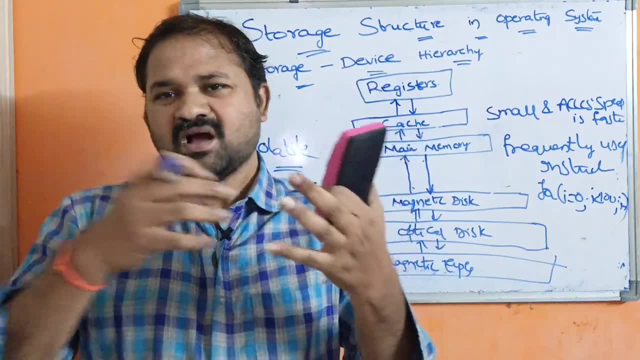 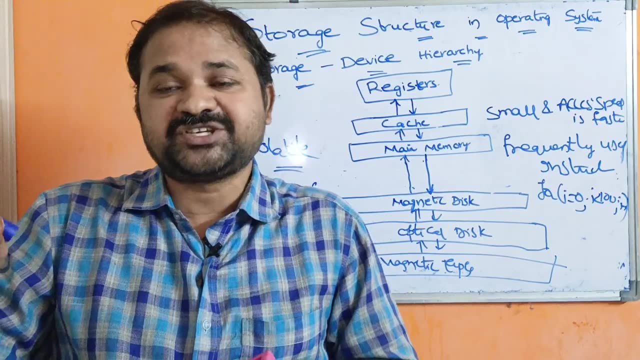 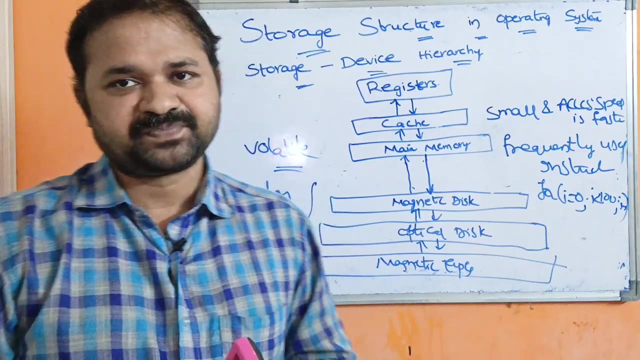 Or if you take any movie, Or if you take any application, After saving that application it will be saved in hard disk only, But whenever we open that application, so whenever we open a game, then that game will be transferred from hard disk into the main memory. 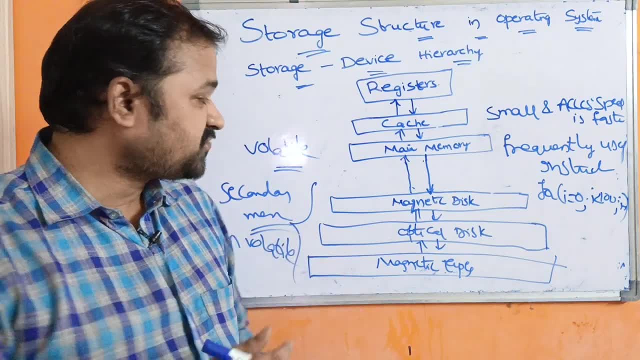 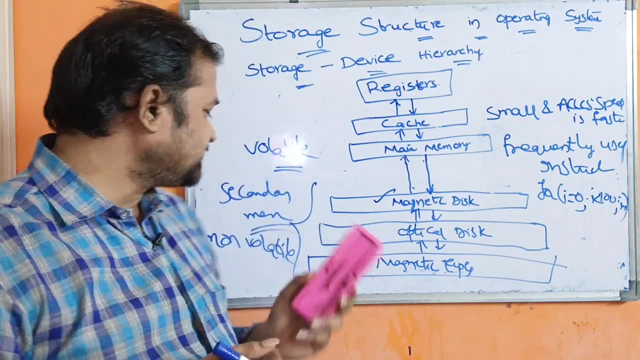 So that is about what is secondary memory. The best examples for secondary memory are magnetic disk. Magnetic disk is nothing but hard disk, So hard disk is the best example for secondary memory. So the next example is magnetic disk. Magnetic disk is nothing but hard disk. 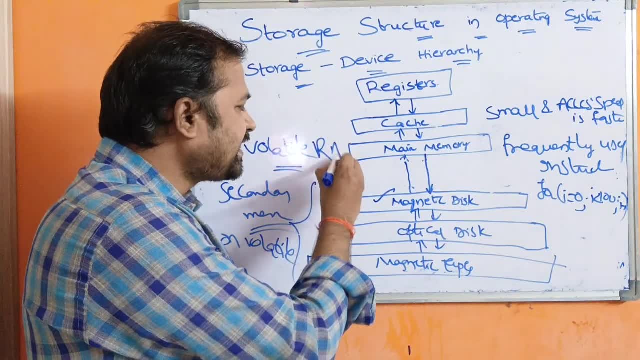 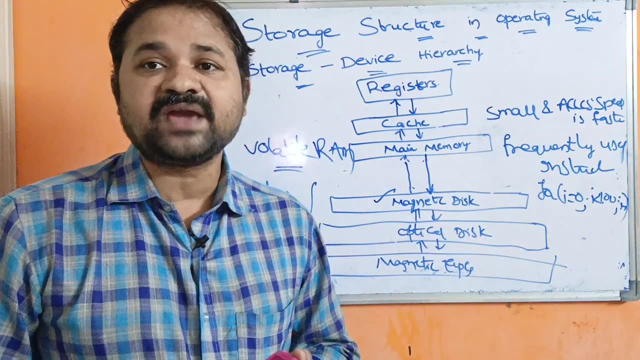 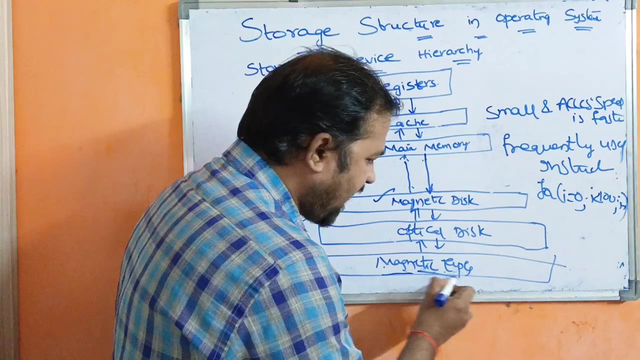 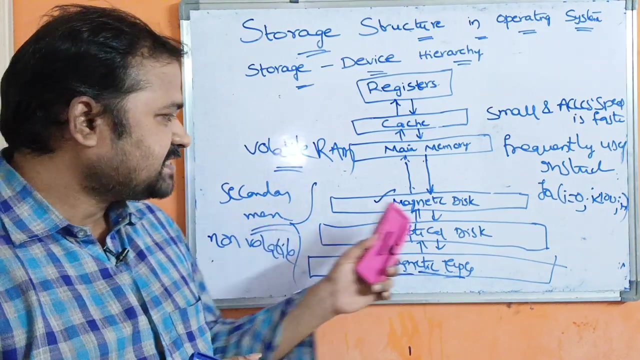 various. the best example for the main memory is RAM. so RAM stands for random access memory. okay, optical disk means floppy drive, CD disks. those are nothing but optical disk. and now let us see about magnetic tape, magnetic tape. magnetic tape is also a secondary memory device. magnetic tape is also just like. 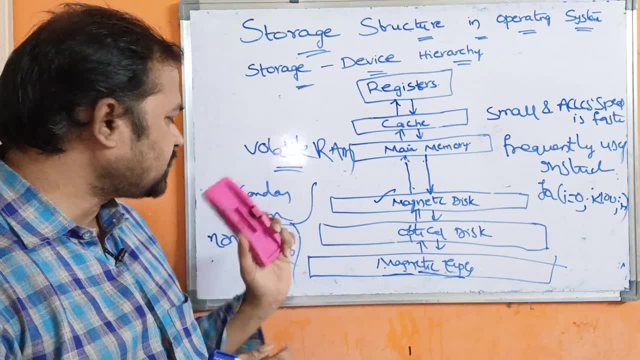 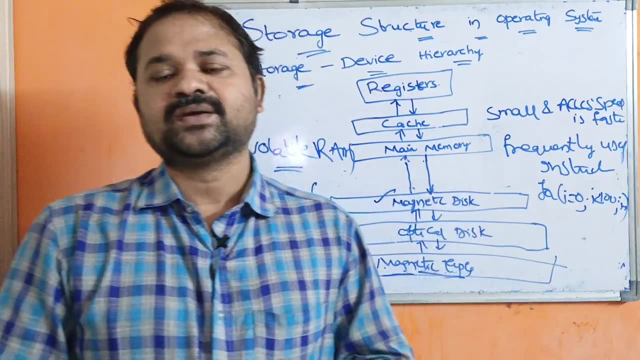 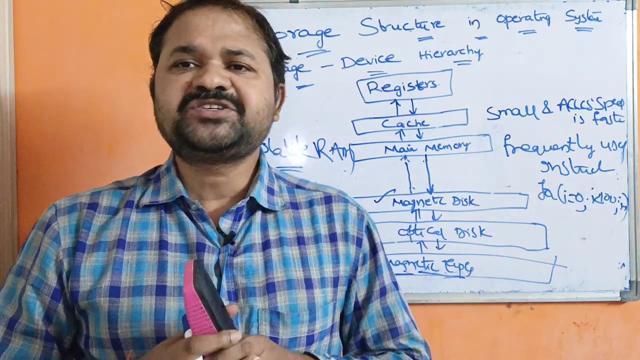 magnetic disk. optical disk. magnetic tape is also a secondary memory device. it is also useful in order to store the information permanently in the computer, but it is used in the olden days. in the olden days magnetic tapes were used. the major problem with magnetic tape is it provides sequential access. it provides 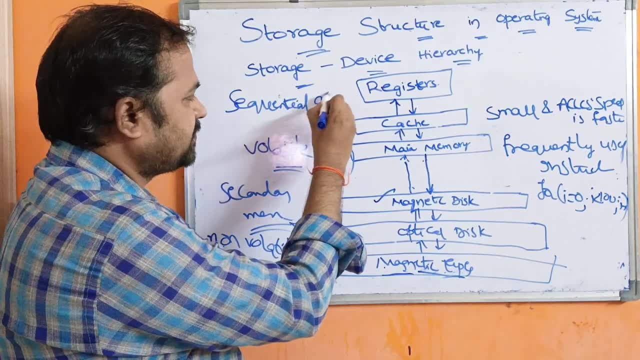 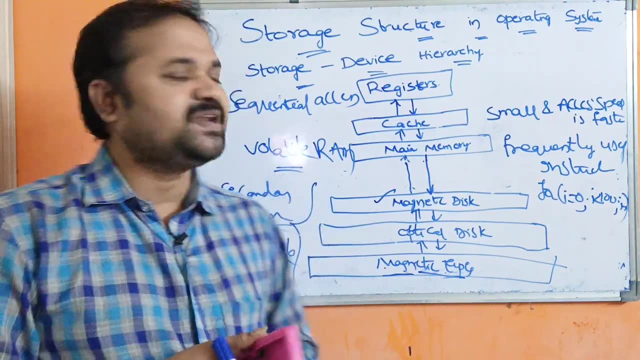 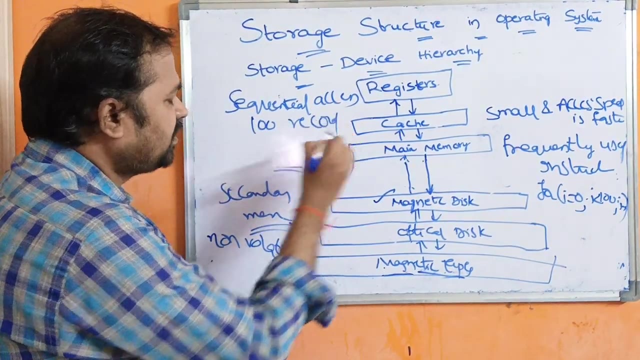 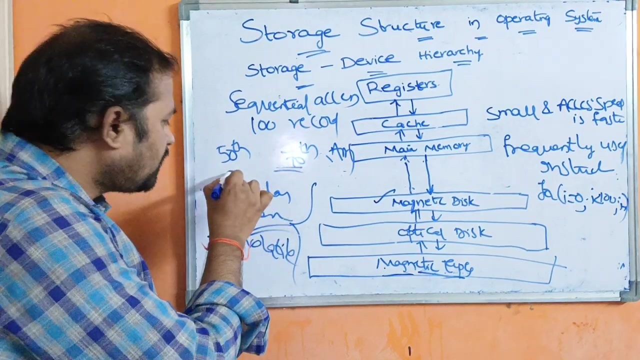 sequential access. random access is not possible, so sequential access means the records will be accessed 1by 1. let us assume that we have a file which contains totally 100 records. so we have a files which contains totally 100 records. assumes that we are yet 50th record and I want to access 70th record. so we now we are. 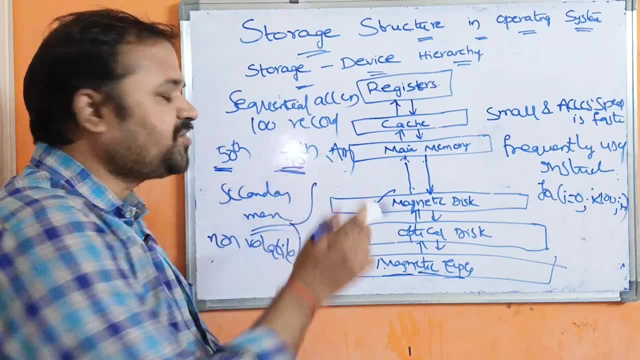 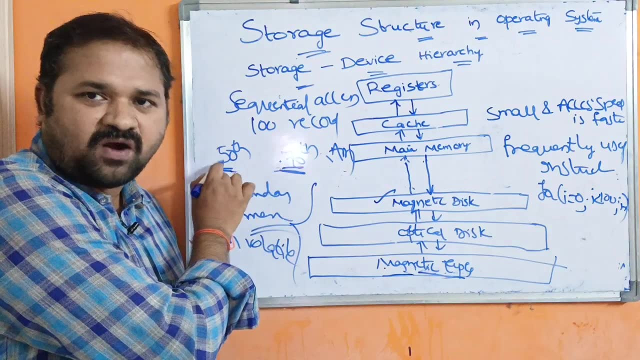 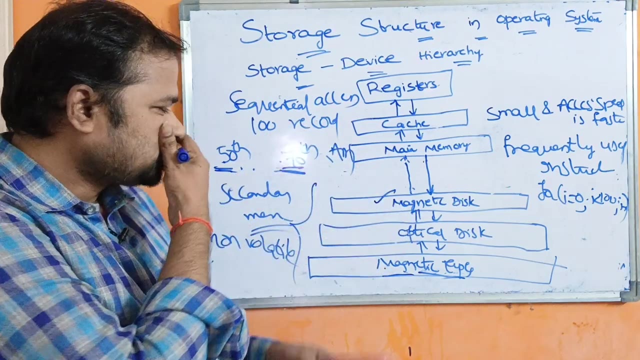 at fifty, 50th record. and what is our target? we want to access 70th record. But the problem with magnetic tape is: all the records will be accessible. so after 50 we need to access 51, after 51 we need to access 52, after 52 we need to access 53. so likewise we have to access all. 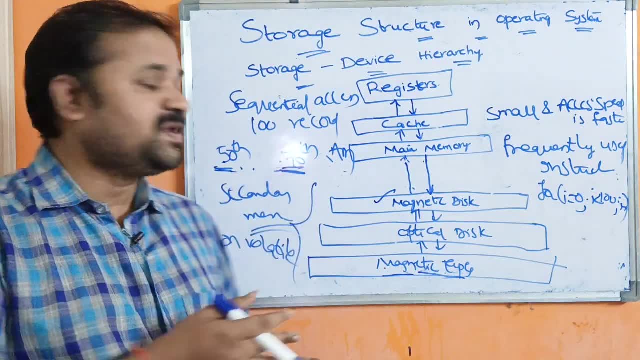 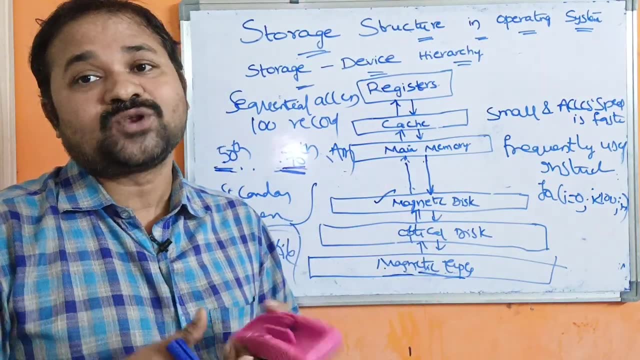 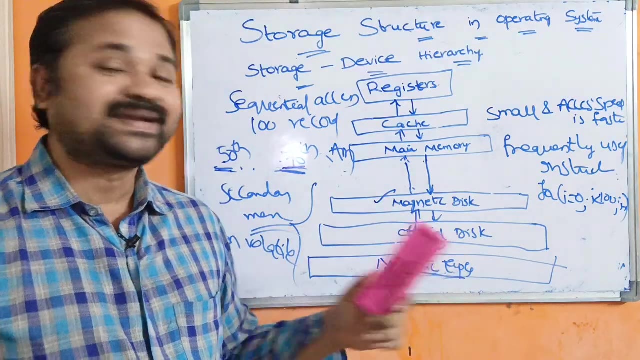 the records between 58 to 70 directly randomly. we can't access 70th record, so this is the problem here. the access speed is very, very, very, very slow here when compared with magnetic disc. magnetic disc is extremely faster when compared with magnetic tape in the olden days, magnetic tapes. 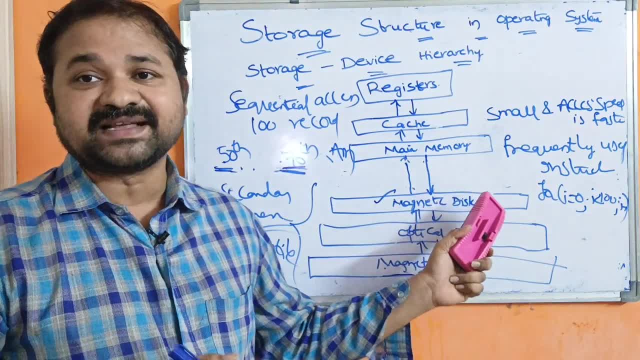 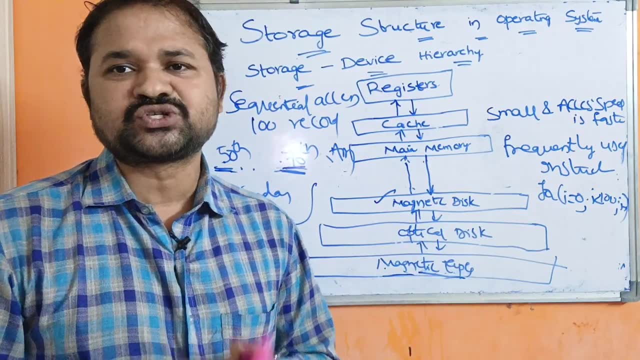 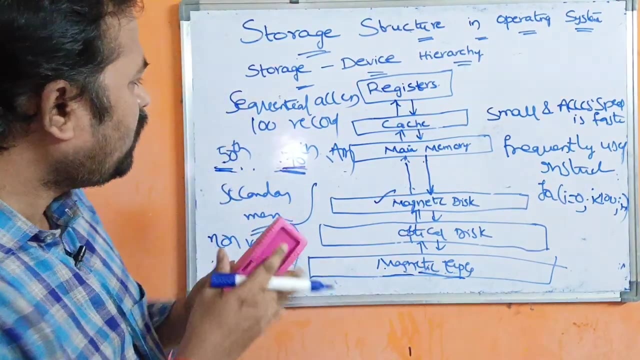 were used, but nowadays we are using hard disk that is nothing but magnetic disk only. we know about cd-rom, compact disc, floppy drive. it is useful in order to store the information permanently in the corresponding disk or in the floppy drive. okay, and now let us see about these devices in terms 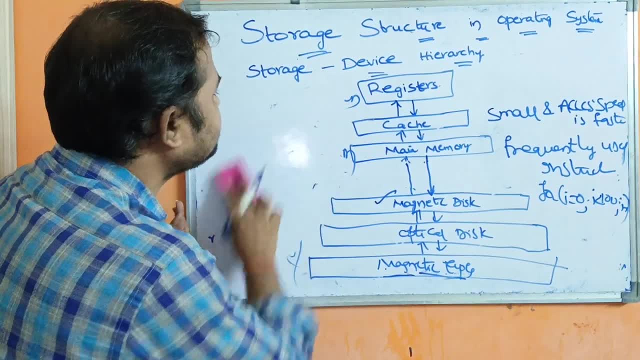 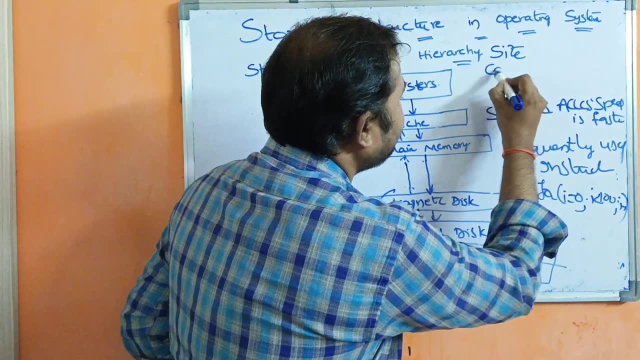 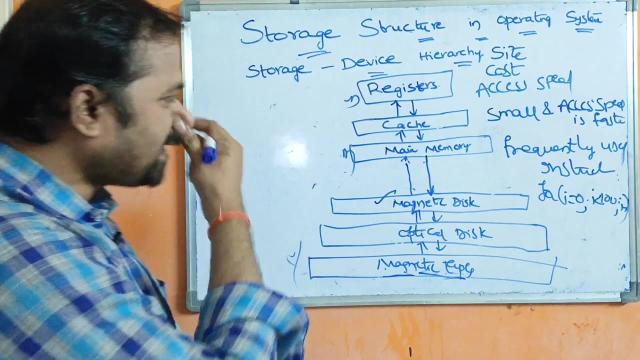 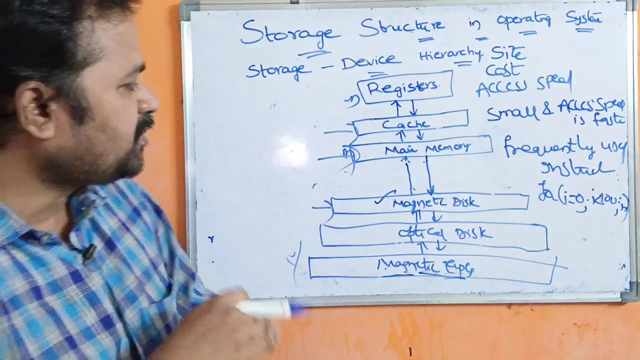 of three properties. in terms of three properties, let us see about these devices. the first property is size, the second property is cost and the third property is access speed. access speed: let us focus on cache memory, main memory and magnetic disk. okay, cache memory, main memory and magnetic. 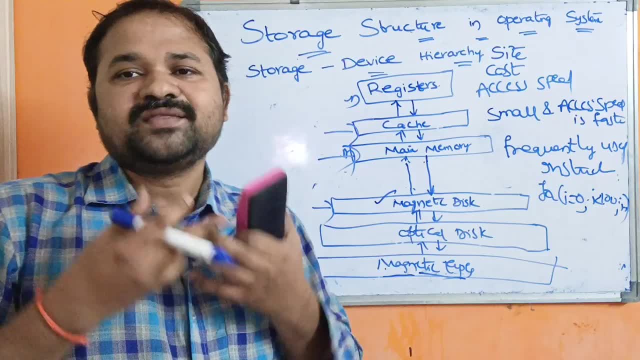 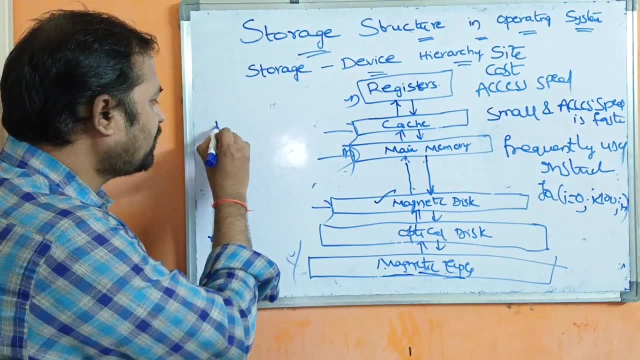 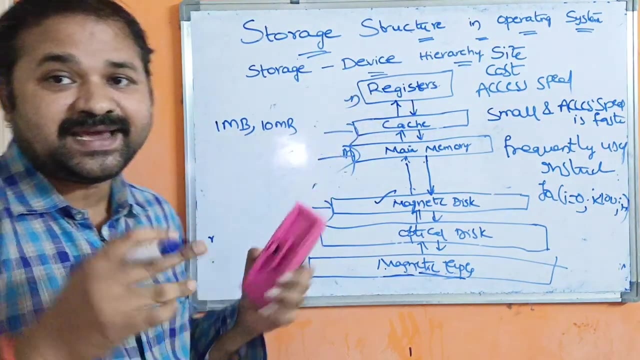 disk. why? because register stores the information in that, now in the form of bits only. okay, here the size of the cache memory will be in the forms like 1mb, 2mb, 10mb. so the size is like this: 1mb, 2mb, 3mb, 4mb, 5mb, likewise, whereas coming to the main memory. 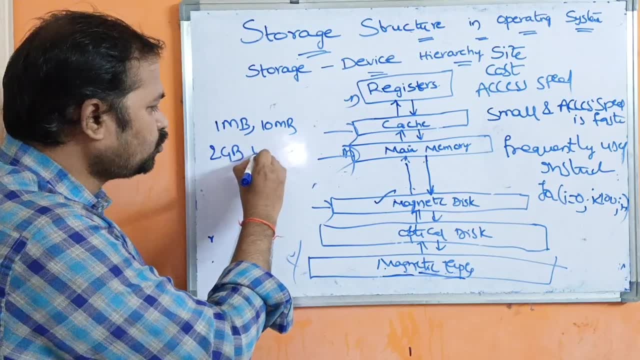 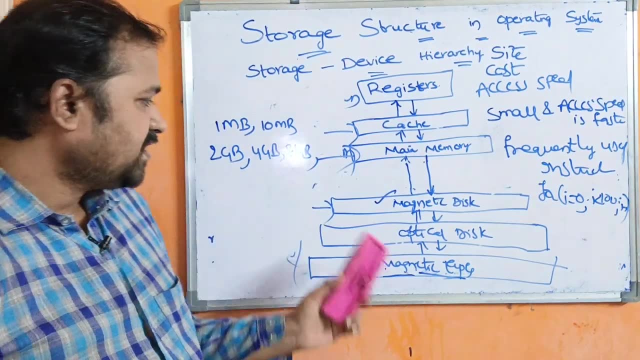 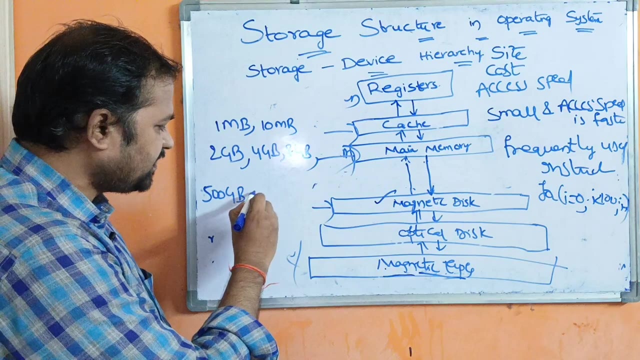 the size of the main memory will be in the form of 2gb, 4gb, 18gb, 16gb, 32gb, 64gb. likewise, whereas the size of the magnetic disk will be in the form of 500 gb, that is, nothing but 200 gb. 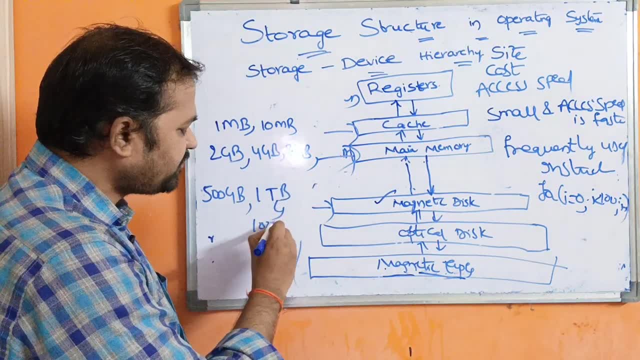 or 1 terabyte. 1 terabyte and the size of the main memory will be in the form of 2gb, 4gb, 18gb, 16gb, 16gb or one terabyte. 4 gb is nothing but 1024 gb. likewise, the size will be like this: now let 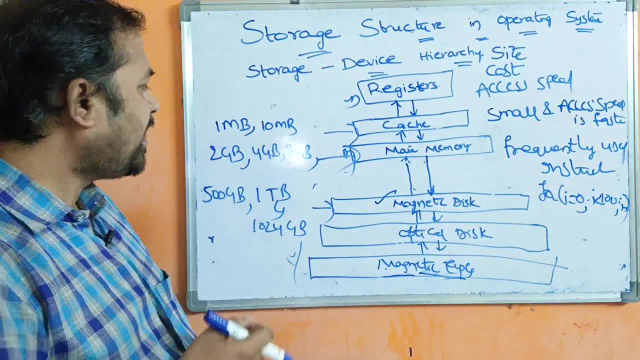 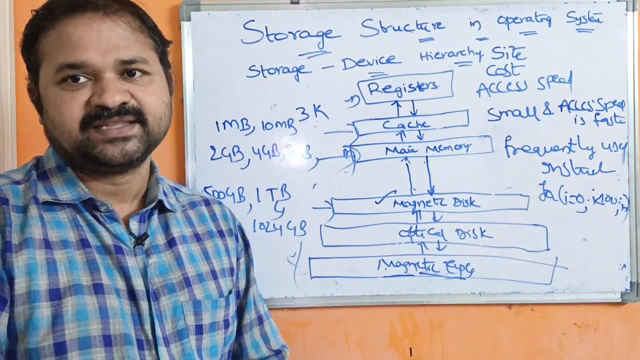 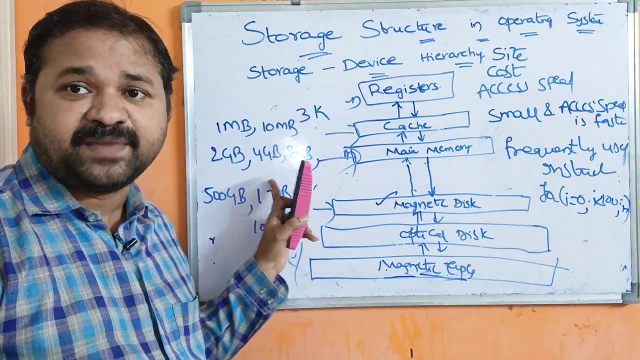 us see about the cast here. in order to buy a 10 mb of cache memory, we need- let us assume that we need some 3000 rupees, three, three thousand, three k three thousand rupees. likewise, in order to buy a 4gb of the main memory- in order to buy a 4gb of the main memory, we need: 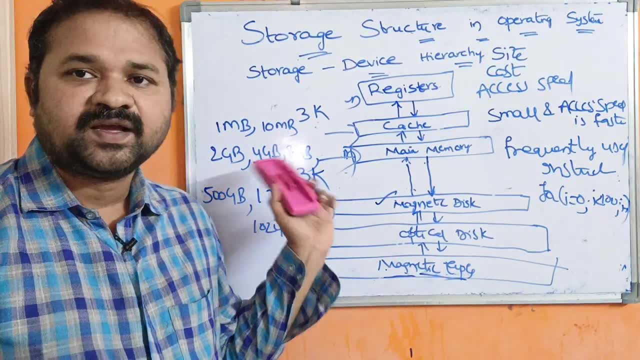 to pay the correct 10gb of the main memory compared to 10gb of the main memory. that is, 4gb of the main memory converted into many extra memory. the process of abdominal attack: 3k rupees in order to buy 4 jb of the main memory. we need to pay 3 kb in order to buy 10 mb of the. 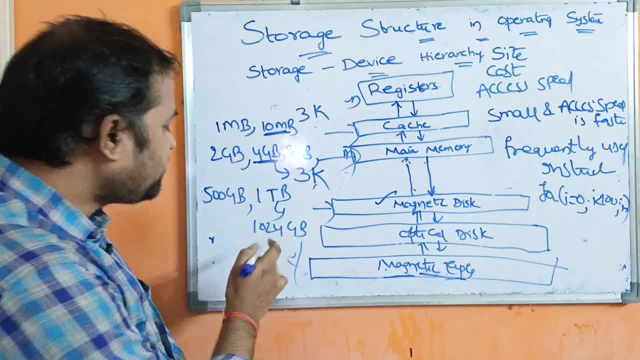 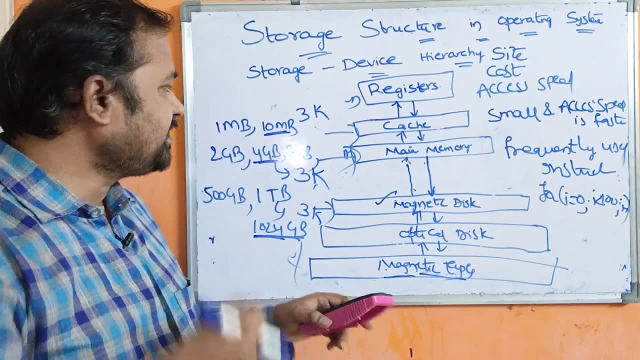 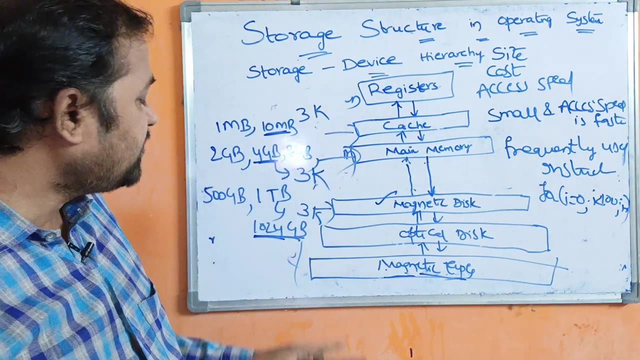 cache memory, we need to pay 3k. so likewise, in order to buy 1024 gb, we require 3 kb- 3000. so here what is the point? here we need 3000 rupees for buying 10 mb of the cache memory, 4 gb of the. 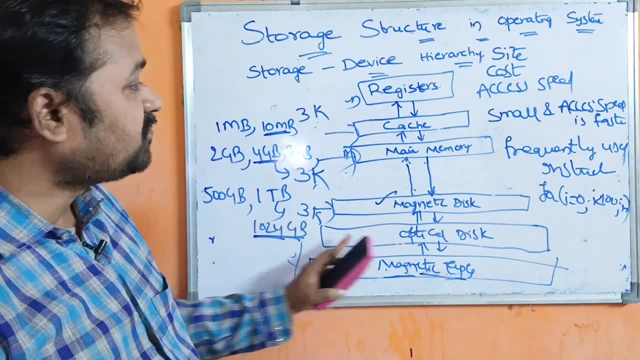 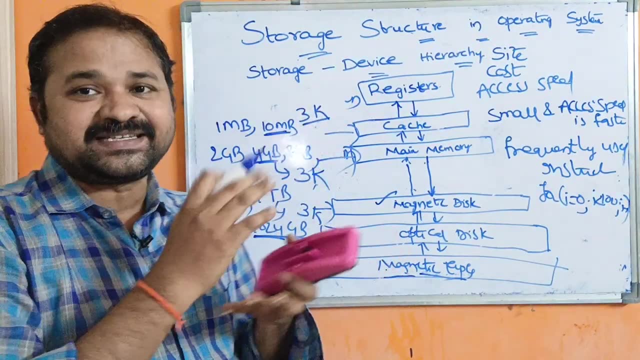 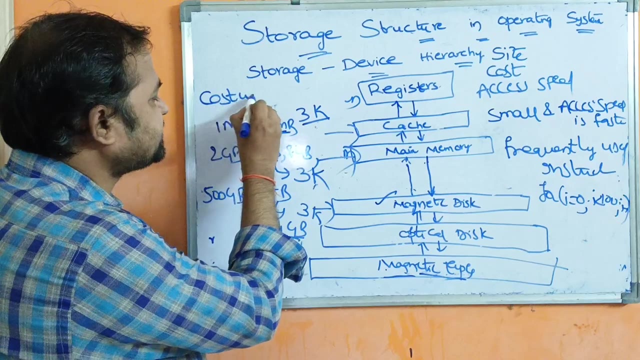 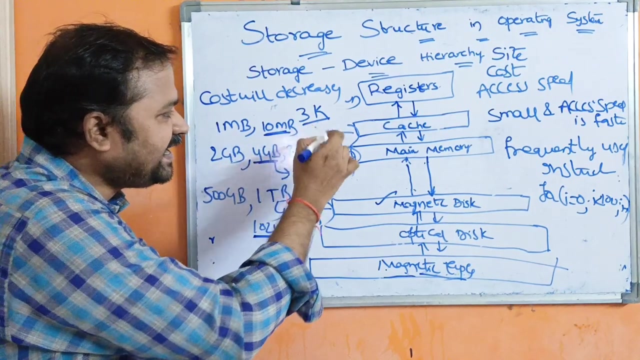 cache memory as well as 1024 gb of the main memory. okay, so here the point is: as the storage capacity increases, as the storage capacity increases, we can say that the cost will decreases. the cost will decreases. so for buying 10 mb of the cache, we require 3k. 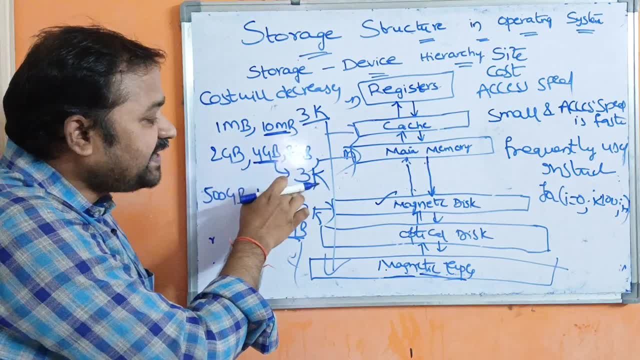 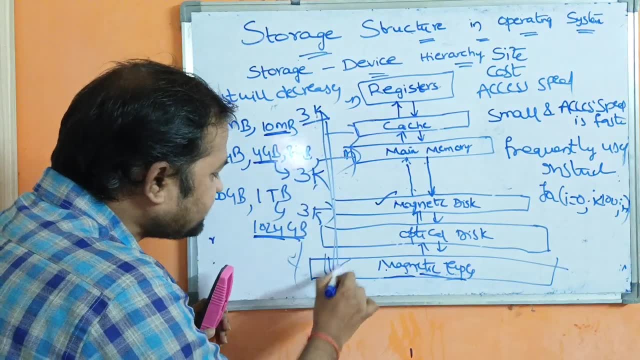 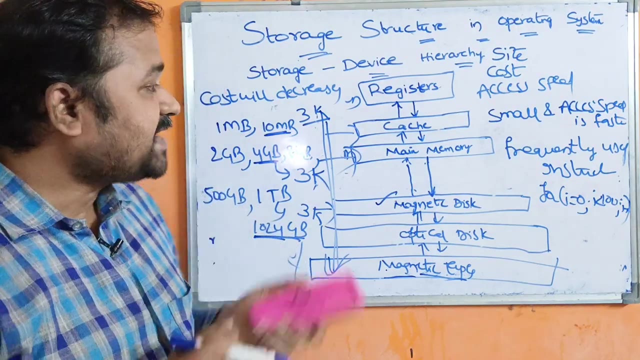 for buying 4 gb, we require 3k. for buying 1024: 4gb, we required 3k. so as the storage capacity, as the storage capacity increases, so we can say that the cost will be decreases. the cost per bit will be decreases as well as. what about access speed? 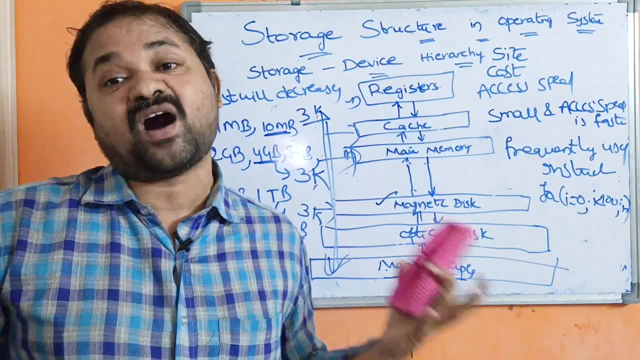 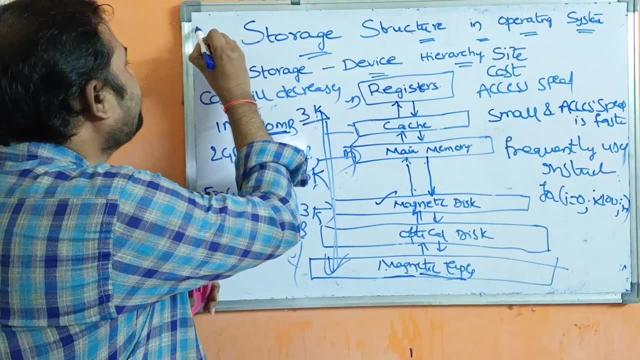 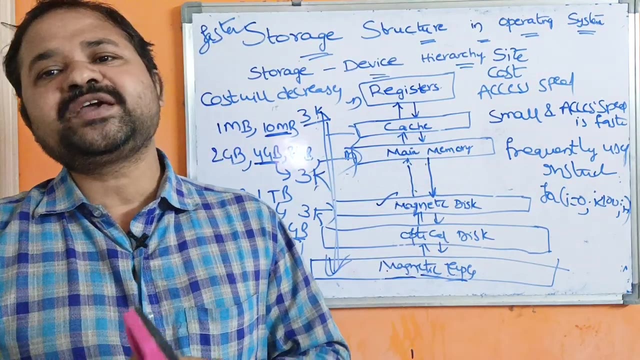 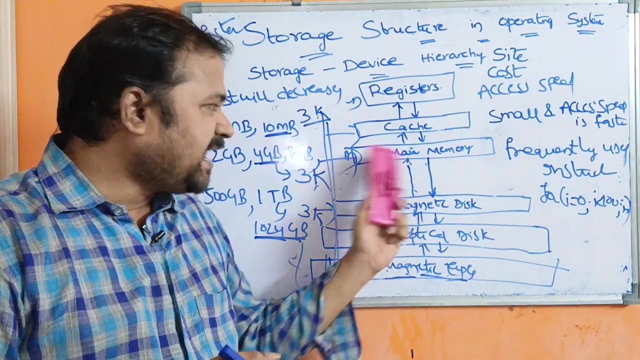 here the catch memory access speed is very, very faster. catch memory is extremely faster than the main memory. so catch memory is very, very faster, very, very faster than main memory. coming to the main memory, main memory access access speed is relatively slower when compared with catch memory, but main memory access speed is extremely faster when compared with hard disk. 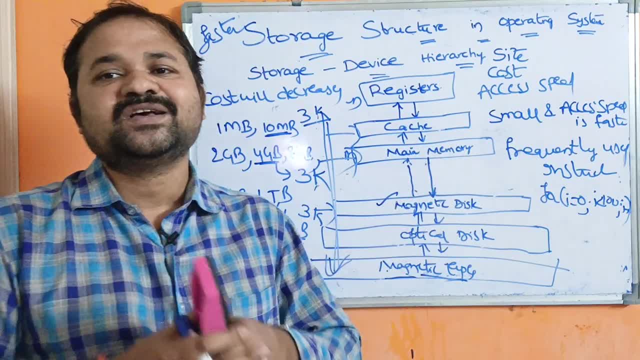 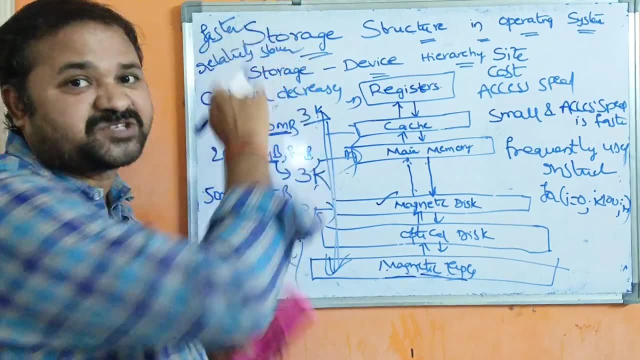 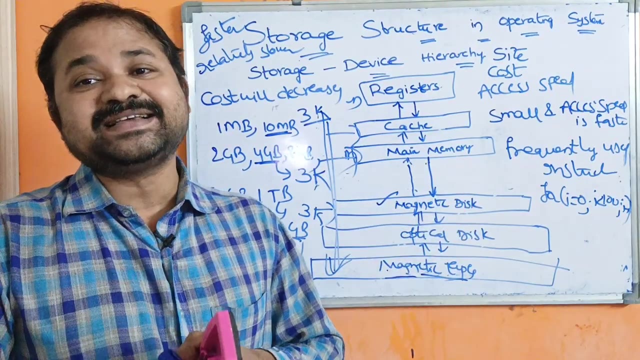 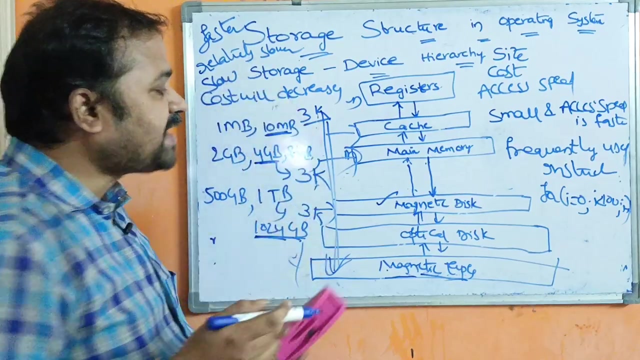 so here, what is the point? main memory access speed is slower, relatively slower, relatively slower when compared with, when compared with catch memory, when compared with catch memory, whereas magnetic disk, magnetic disk is access speed is very, very slow. magnetic disk access speed is very, very slow when compared with main memory, as well as